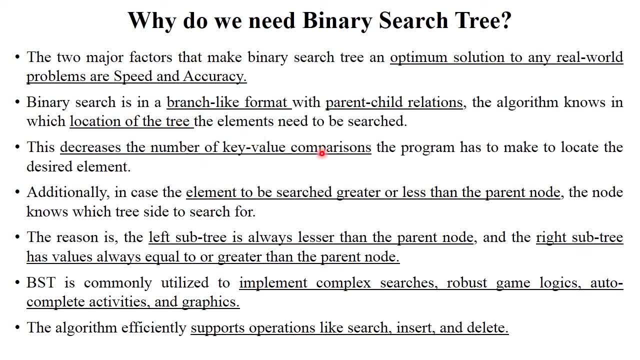 in the tree. This decrease the number of key value comparisons because binary tree stored all the elements in particular order. That's why number of key value comparisons are decreases. The element we search greater or less than the parent node. the node knows which tree. 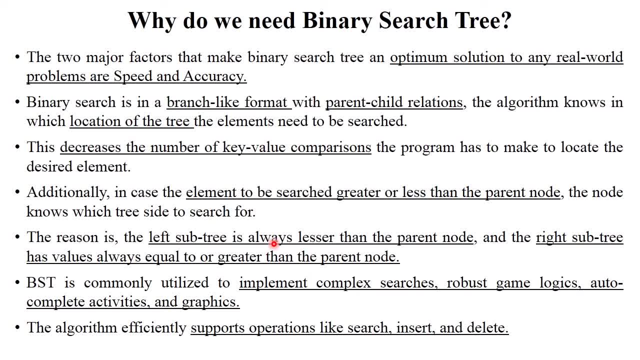 side to be searched: right, because left subtree is always lesser than parent node and right subtree value is always greater than the parent node. This is the concept of binary search tree. Binary search tree is commonly utilized to implement complex search, robust, game logic. 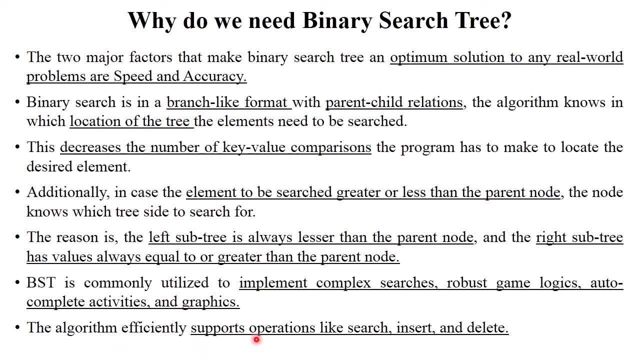 autocomplete activities and graphics. The algorithm efficiently supports operations like search, win and save. You can see the results of binary search tree, dizer that you insert and delete. so binary search trees: advanced algorithm to search a particular data in optimum solution. right, that's why we use or we implement. 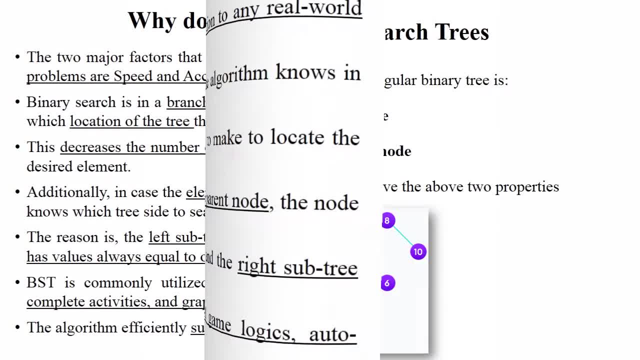 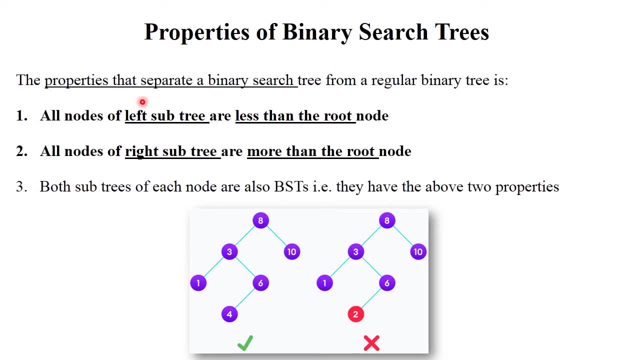 a binary search tree. next now, what exactly binary search tree means, or the properties of binary search tree, the properties that separate a binary search tree from regular binary tree. these are the property. first, all nodes of left subtree are less than the root node and all nodes of right subtree are more than. 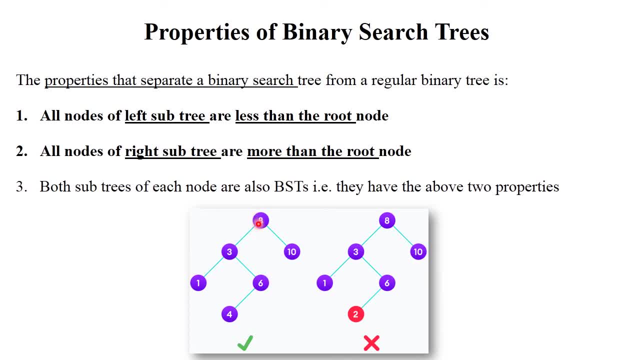 the root node. say, in this diagram, the root node is eight right, so three is less than eight and one is less than their parent node. that is three right, and six is greater than three and also less than eight. okay, so left subtree stores all the less value than the root node. 1, 3, 6, 4, these are the lesser value than the root node. 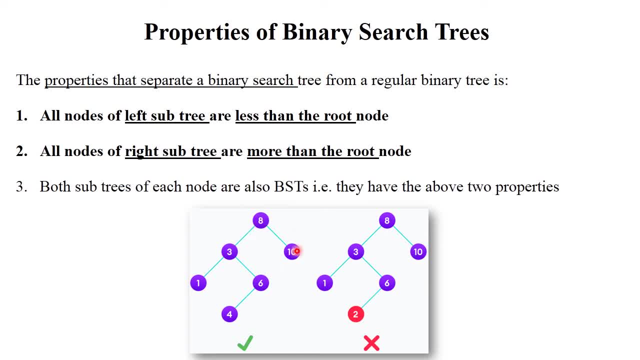 and 10 is greater than the root node- clear. So this is the concept of binary search tree and both the sub tree of each node are also a binary search tree. This left sub tree also follow binary search tree property and right sub tree also follow binary search tree property. 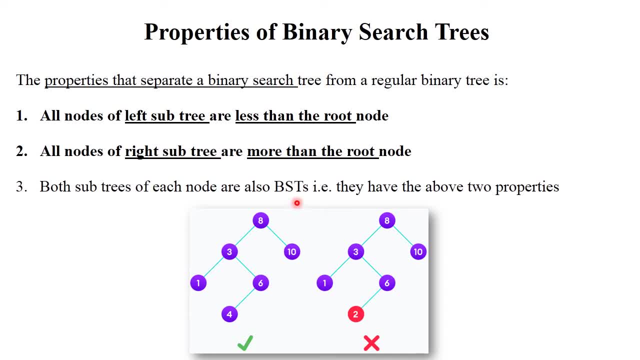 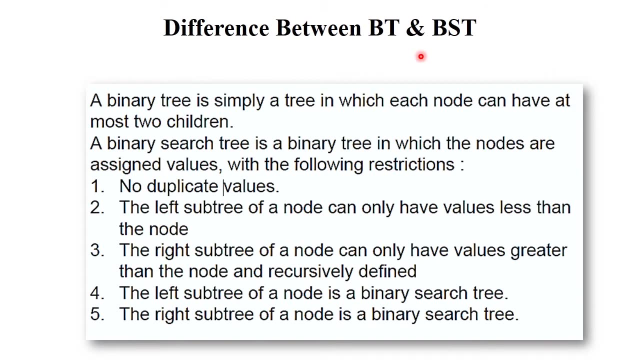 ok, So this is the concept of binary search tree: Left sub tree- less value than root node and right sub tree- more value, greater value than root node. clear next, Now the difference between binary tree and binary search tree. A binary tree is a simple tree. each node can have at most two. 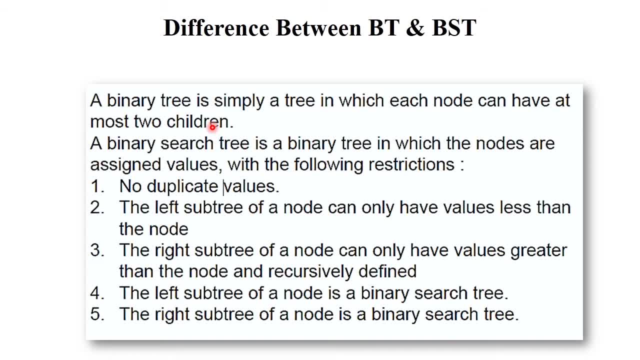 children, right, We will learn this binary tree concept in my last video, right? So binary tree simply means, at most, two children. but a binary search tree is a binary tree in which nodes are assigned value with following restrictions: They have some restrictions or proper rules for implementation. 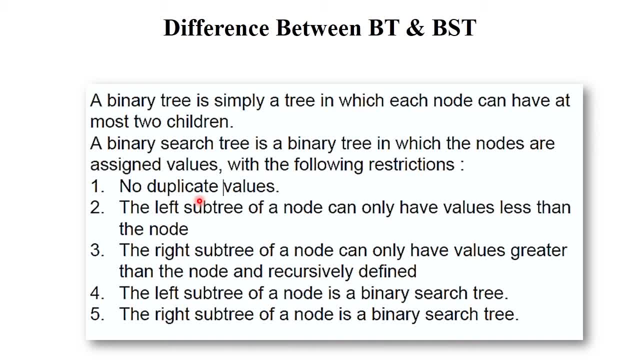 of binary search tree. The first: no duplicate values. the left sub tree of node can only have values less than the root node. The right sub tree of values greater than the root node and recursively defined. ok, So left sub tree of node is also a binary search tree and right sub tree of node is also a binary search tree. So this is the concept of binary search tree, clear. next, 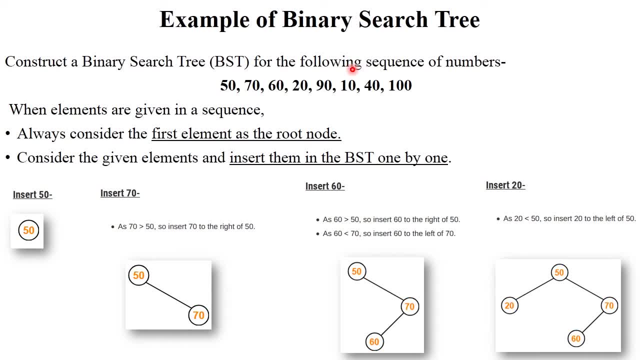 Now the example of binary search tree. First I'll explain the example Soов it's easier to understand the operations of binary search tree. So the given example is: construct a binary search tree in following sequence of numbers The particular sequence is given With element. are given in sequence toㅠㅠ: always consider the first element is root node. 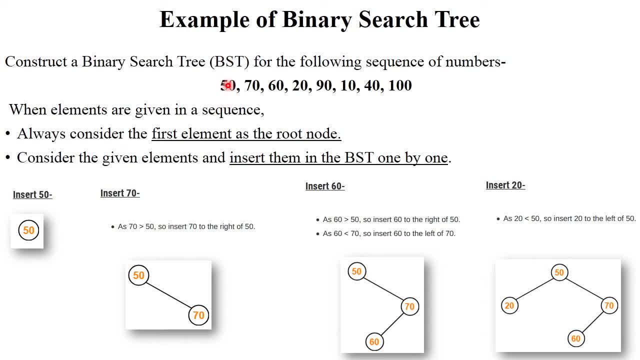 Always consider 3 button, JSON andwen serial kernel Wild node. always consider the first element is your root node. okay, and insert them in binary search tree one by one. so see here: the first is 50, so insert 50, the one node is created and this node 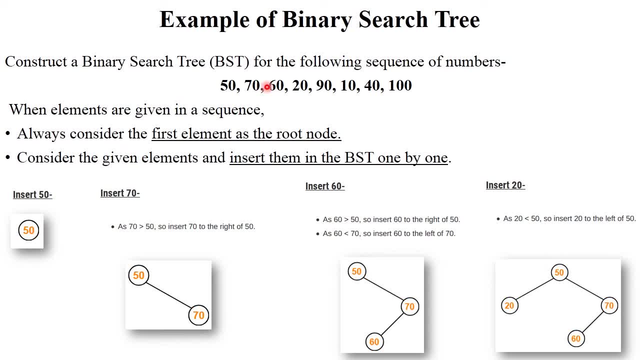 is called as root node. okay, according to this sequence, we will implement a binary search tree. next 70. now compare 70 with this root node: 70 is greater than 50. greater value on right side and less value is on left side. okay, next 60. again, 60 is greater than 50 and 60 is less than 70. so it 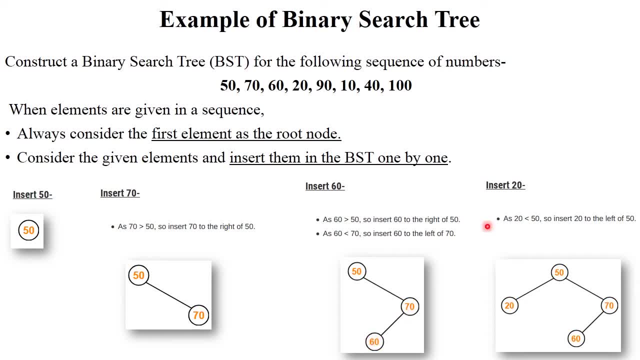 goes to left side of 70, next 20, 20 again, compare with the root node, 50 always comparison. start with the parent node or the root node. okay, level by level you should compare the particular value level by level. so 20 is less than 50. it goes to left side. 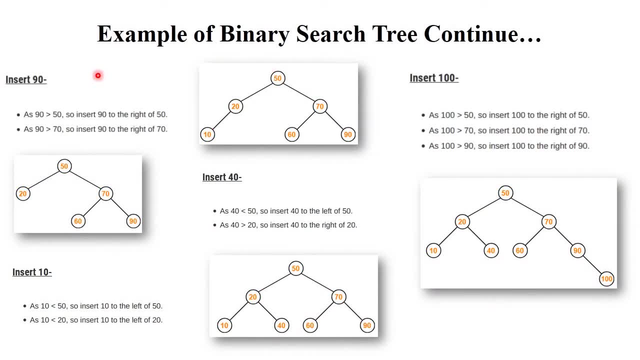 clear. next the next insert: 90. 90 is greater than 50. it moves to right side. 90 is greater than 70, again move to right side. clear. next insert 10: 10 is less than 50. move to left side again. 10 is less than 20. 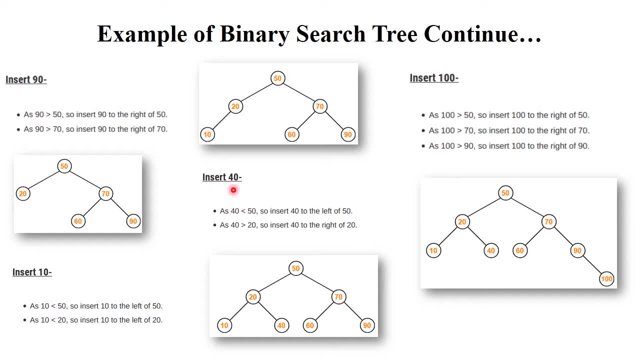 move to left side. clear next 40. now check: 40 is less than 50. so it goes to left side. now compare 40 with 20. 40 is greater than 20. if it is greater, move to right side. right next last 100. again compare: 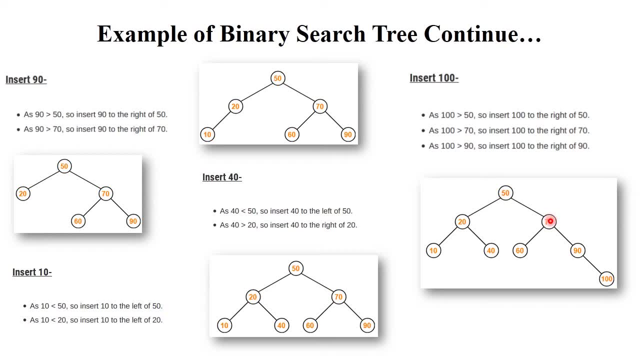 100 with 50. 100 is greater than 50, move to right side. 100 is greater than 70, move to right side again. 100 is greater than 90, move to right side. clear, then insert node here. so this is the concept of binary search tree: less value on left. 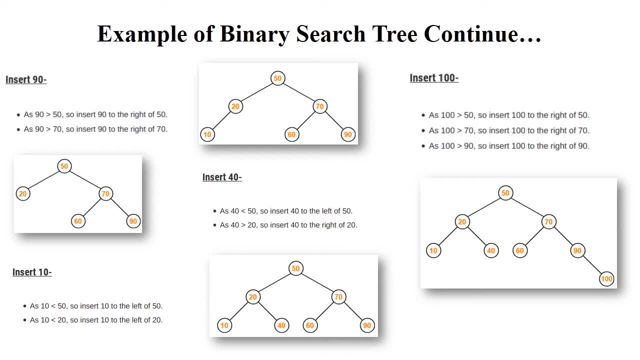 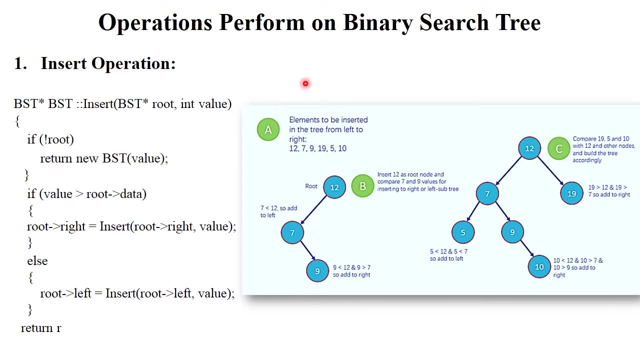 tree: right value on right sub-tree: Clear Next. now the next operations perform on binary search tree, So it's very easy to understand. The first operation is insert operation. See in this diagram. the given sequence is 12, 7,, 9,, 19,, 5 and 10.. Okay So. 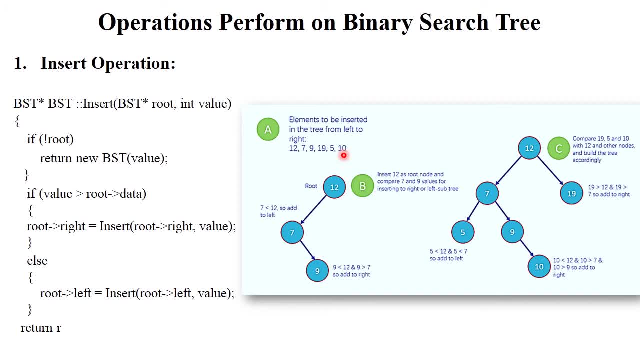 how to insert the elements. I already explained examples in previous slide. Similar way, you should insert the binary search tree value. Okay, So first value is considered as the root node, that is 12.. Okay, So 7.. 7 is less than 12.. So add on. 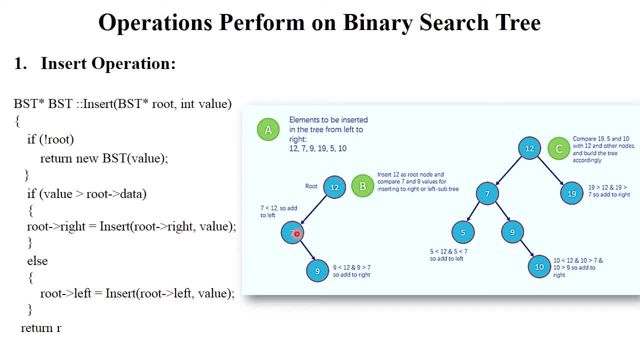 left side, Next 9.. 9 is less than 12, but greater than 7.. So add on right side. Okay, In this way, remaining elements are added into the binary tree, Clear. So this is one of these things: simple logic of insertion. Now, this is the pseudo code, or we can say algorithm of insertion. 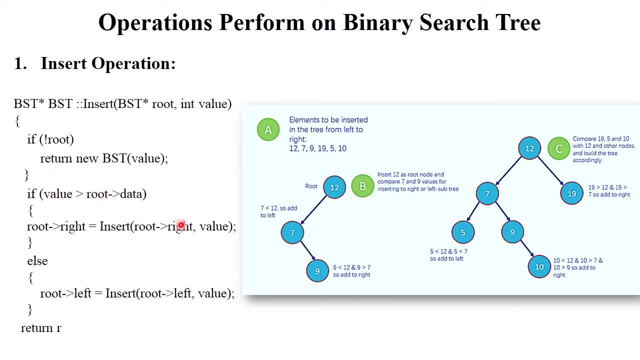 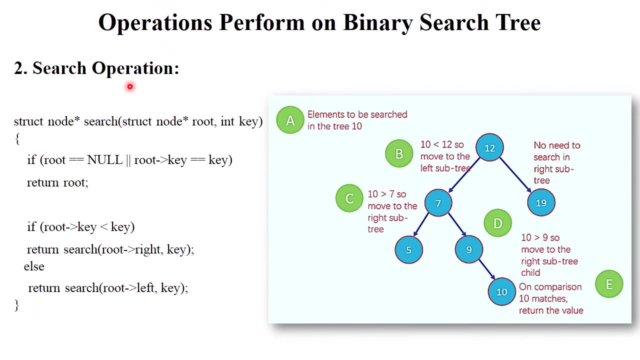 If value greater than root, then insert on the right side, else insert on left side. So this is the logic of insertion function. Clear Next. Now the next operation is search operation. Search operation also use same logic as insertion operation. See, this is your given binary search. 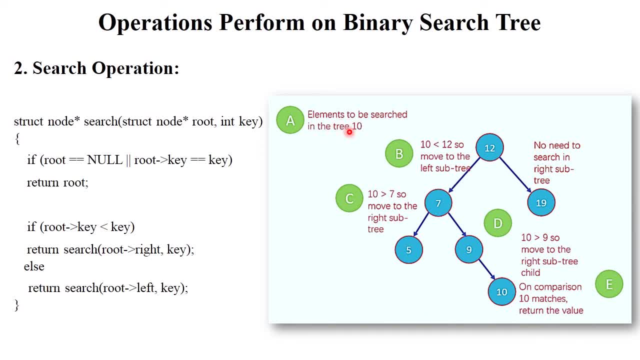 tree. Ok, Now elements to be searched in the tree 10.. You should search the element 10 in this given tree. Ok, So first compare 10 with 12.. 10 is less than 12. move to left side Now. compare 10 with 7.. 10 is greater than 7. Right, So move to right side Again: 10. is compare with 9.. 10 is less than 7.. Right, So move to left side Now. compare 10 with 7.. 10 is greater than 7.. Right, So move to right side Again. 10 is compare with 9. 10. 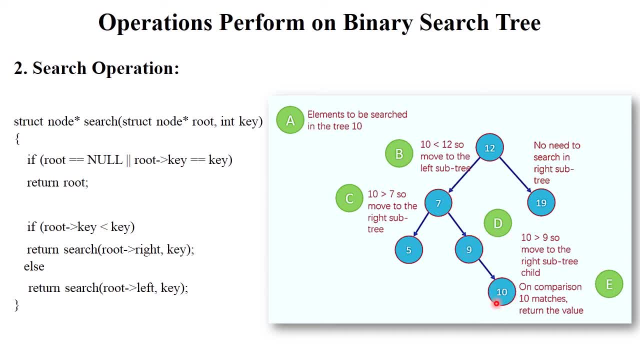 is greater than 7.. 10 is greater than 7.. Right, So move to right side And here on comparison, 10 matches, So they return the value 10.. Your location is in this particular place, Clear. So this is your search operation. Search: always start with parents to leaf node. 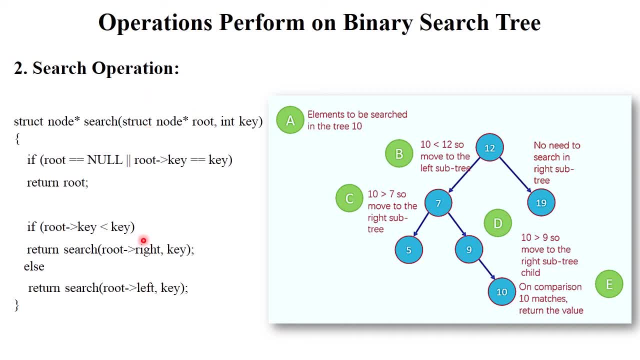 Ok, In between that And this is the logic of search operation. If root equal to null or root of value is exactly equal to search value, For example if you want to search for 12.. So at that time 12 is match with 12 or the root value. Right, So is return the root. 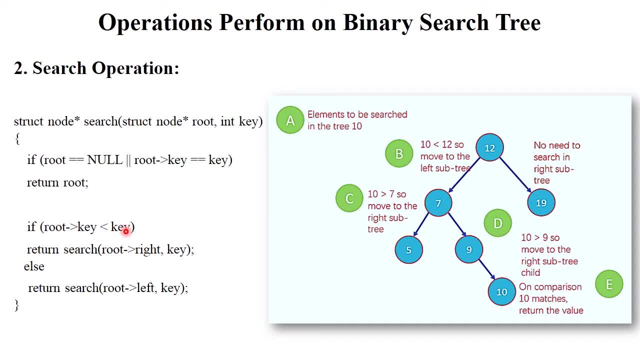 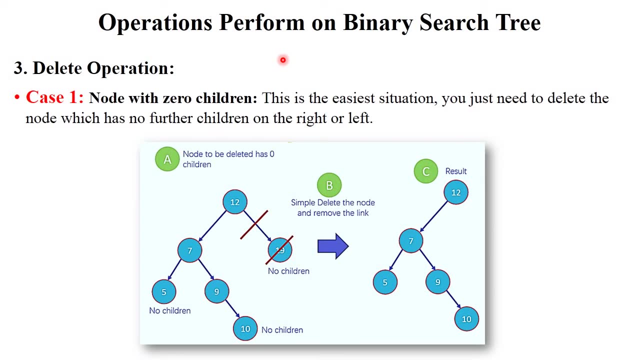 Otherwise, again, root value: check whether it is less than goes to right side, greater than right side and less than goes to left side. Clear. So this is the concept of search operations. Next, Now, the next operation perform on binary search tree is delete operation. So delete. 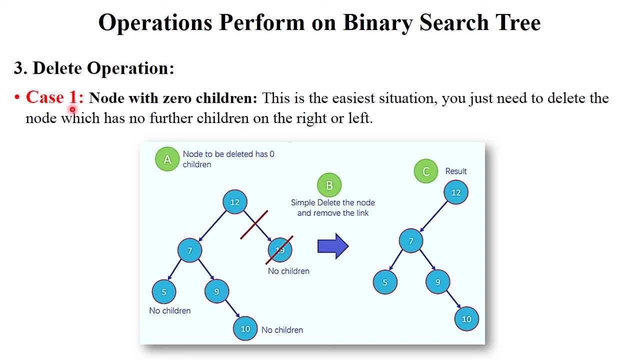 operation has total 3 case. Let's see first case, Case 1.. Node with 0 children. This is your first case. Ok Means you should delete the node which has 0 children. So this is the easiest solution. You just need to delete the node which has no further children. on: 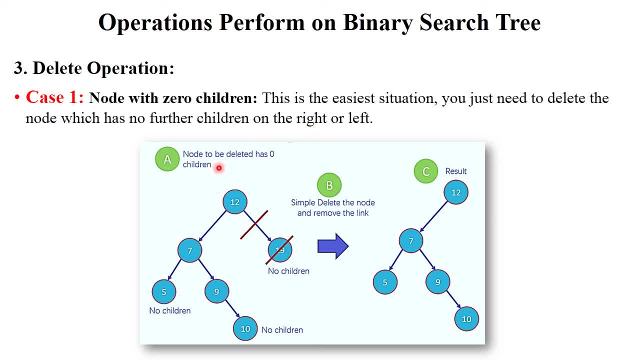 the right or left. See in this diagram: Node to be deleted has 0 children. Ok, Suppose you want to delete a 19.. 19- you want to delete. 19. you want to delete 19- you want to delete. 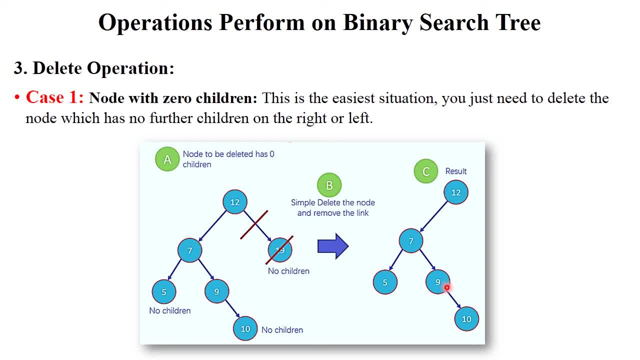 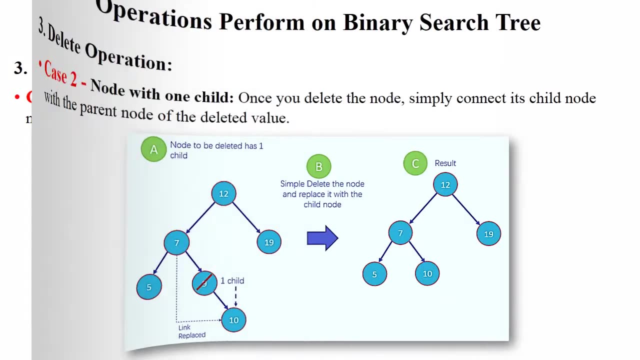 20, you should directly delete it, And this is your remaining tree, Ok, Means, after deletion, this tree will be generated Clear. If there is no children, you should directly delete it, And this is your remaining tree, Ok, Next. Now the second case of delete operation is: 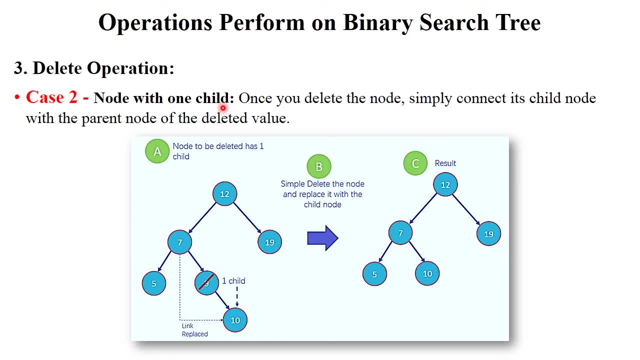 Node with 1 child: Ok. In last case, node with no children. and now the second case is node with 1 child, right? So once you delete the node, simply connect its child node with the parent node of the deleted value, See in this diagram. now you want to delete the node which has one child, ok. So 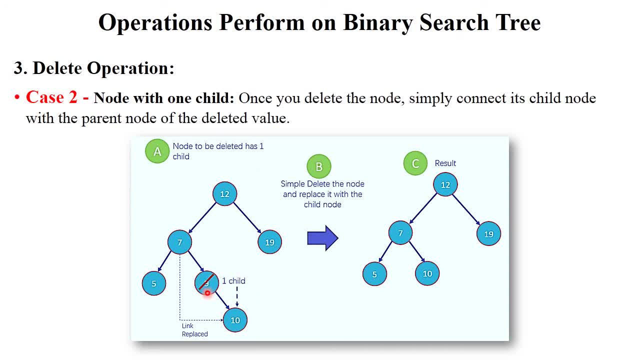 suppose you need to delete this value, that is, 9, node 9. ok, Now, after deletion, deleted this value, this 10 and this 7 will be connected with each other. ok, So this child node is connected to the deleted node's parent node, right, What is? the parent node of 9 is 7 and child is 10.. So 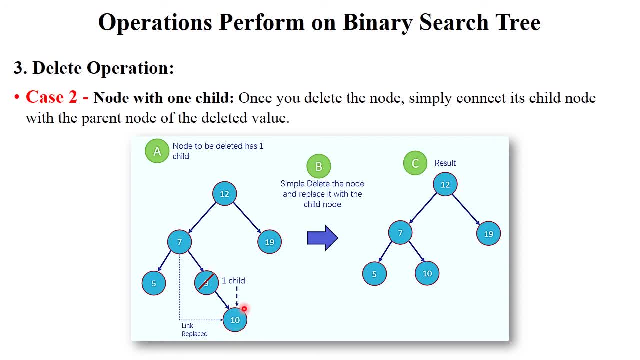 this parent and this 7 are connected with each other. clear. So after deletion, the tree will be generated in this way, that is, 7, 5 and 10 placed as 9th location. clear. So parent and child of deleted node are linked with each other. clear. So this is the concept of second. 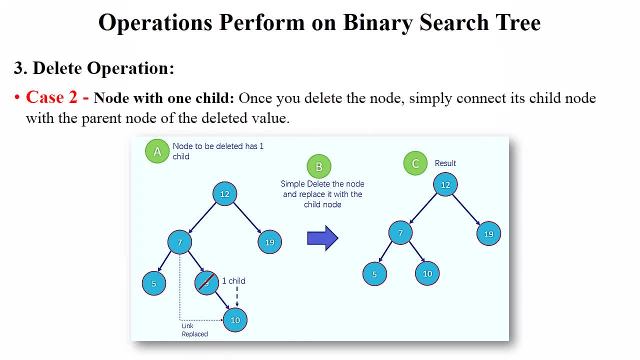 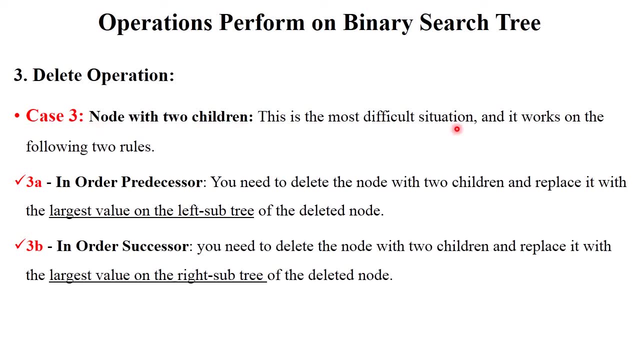 case node with one child. next Now the next third case node with two children. ok, So this is the one of the most difficult situation. It works on the following two rules. It has two rules. The first rule in order predecessor: In this case, largest value of left subtree will be replaced, and second, 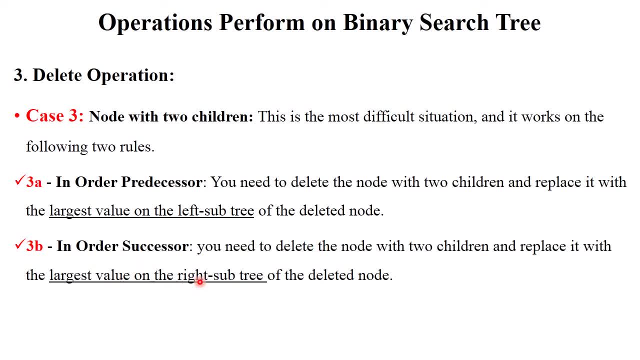 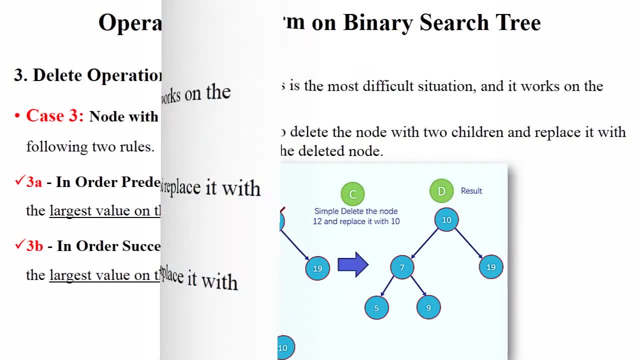 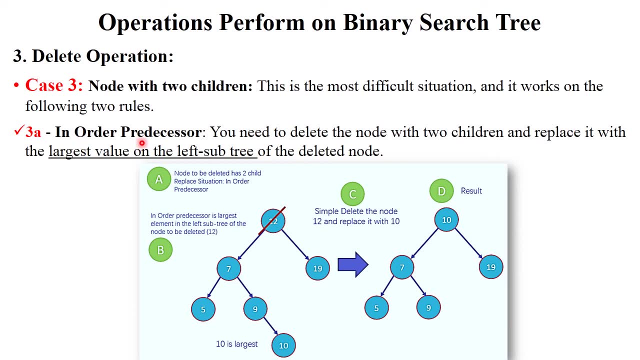 in order: successor, that is largest value on right subtree, will be replaced with deleted node. Let's see with this example Next. Now see here in third case: node with two children. The first rule is in ordr predecessor. See in this diagram: node to be deleted has 2 child. 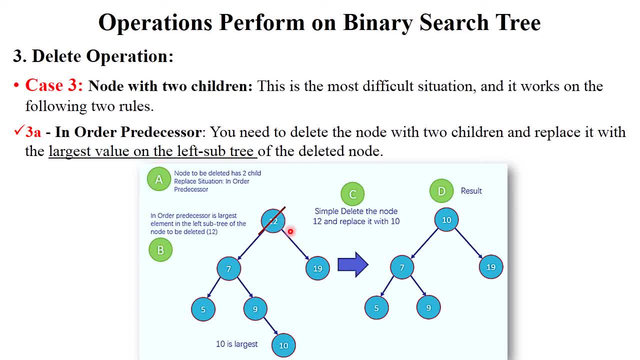 ok, Suppose you want to delete 12.. 12 has two child right. So by using in order predecessor, you should delete this node. In order predecessor means to find out largest value in left sub-tree. ok, you should delete 12. this is your left sub-tree and this is. 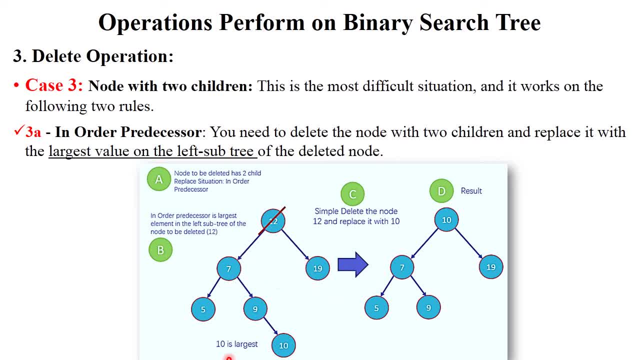 your right sub-tree. ok, now the find out the largest value in left sub-tree, which is the largest value: 10, right, so this 10 is replaced with this deleted node. so 10 goes to at the root place, that is, 12 place. simply replace it, ok, and this is. 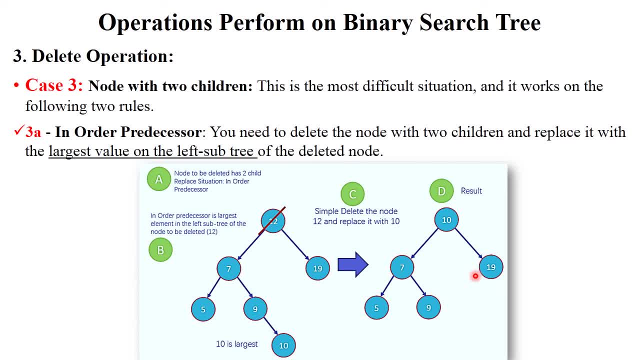 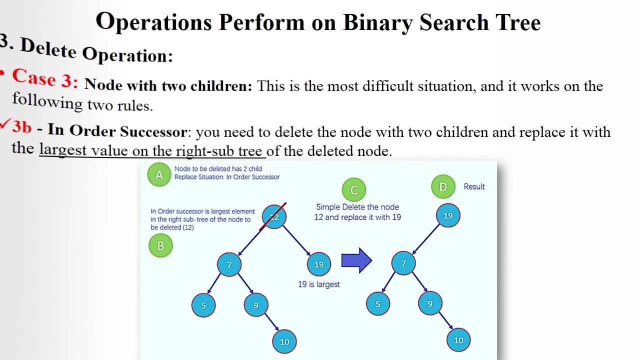 your after deletion node regenerated tree: clear. in in order predecessor: find out largest value. left sub-tree and largest value is replaced with the deleted node clear. this is your first rule. in third case, next now, the second rule is in order successor. now again, suppose you should delete a 12 by using. 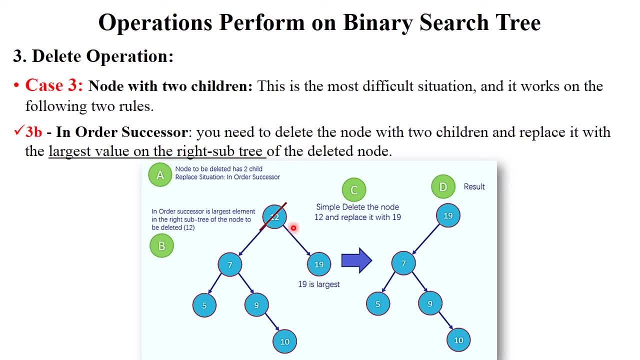 the concept in order successor. in order successor means find out largest node in right sub-tree- ok. predecessor means largest node in left sub-tree and successor means largest node in right sub-tree- ok, so in right sub-tree there is only one node, 19, so it become a largest node right. so this 19. 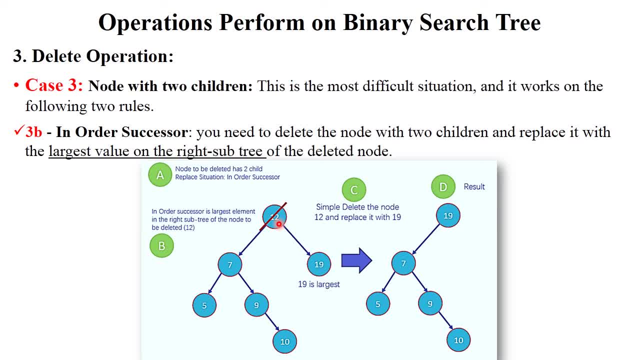 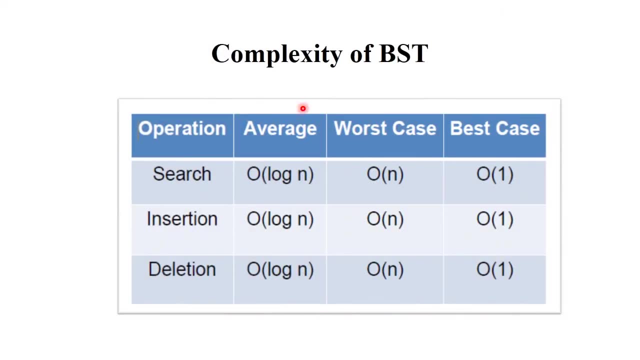 value replaced with this deleted node, that is 12. so after deletion, this tree will be generated clear. so this is the concept of deletion operation in binary search tree. next now, the complexity of binary search tree. so this is the average, worst and best case time. complexity of the binary search tree. algorithm for search. 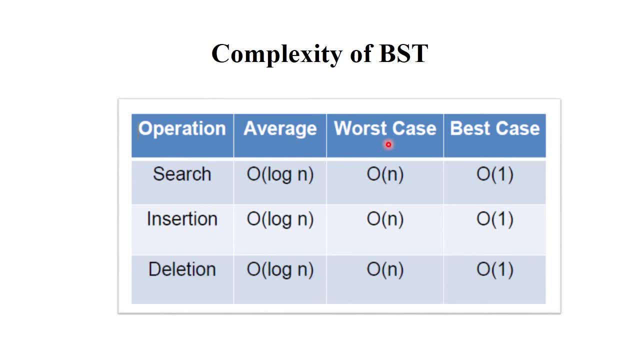 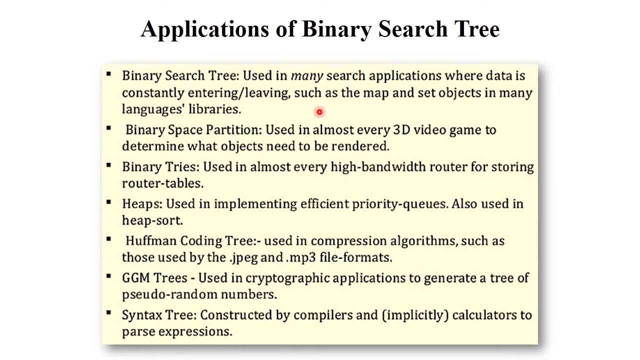 insertion and deletion. average big O log n. worst case big O n and best case big O one. this is the time complexity of binary search tree algorithm clear next. next, applications of binary search tree where we use binary search tree consent. binary search tree used in many such application. 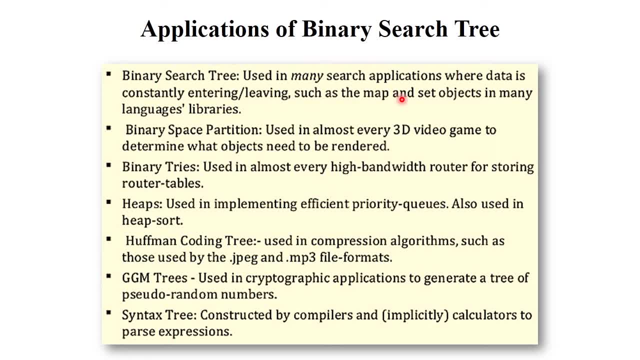 their data is constantly living or enter 18kn Roccata object in many language library. binary search tree concept used binary space partition. it used almost every 3d video game to determine what object need to be rendered right in 3d video game: football striker in said field州. it used almost every high